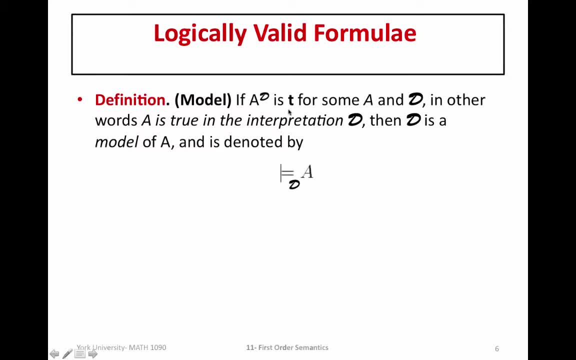 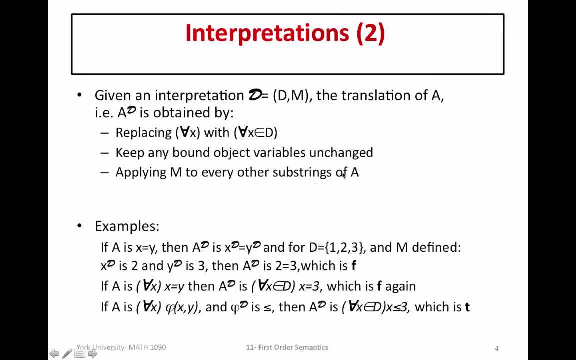 A is a model for that well-formed formula A, if it makes it true. So, for example, in our previous video, our specific model, our specific interpretation with domain D and translator M for this well-formed formula for all- x, phi, x, y- was true. 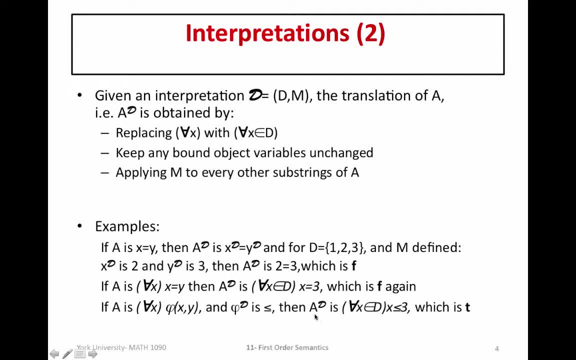 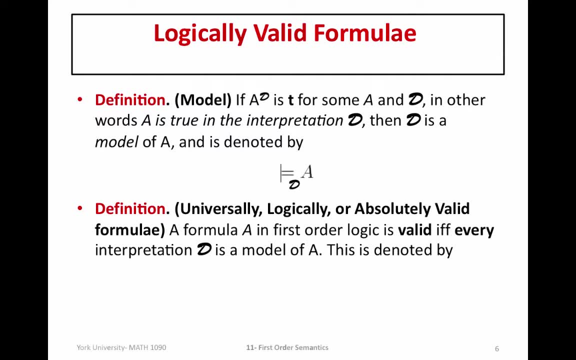 So in this case, this interpretation is a model of this well-formed formula. In addition, a formula A in first order logic is said to be valid either universally logically or absolutely valid if, and only if, every interpretation D is a model of A. So this means if every. 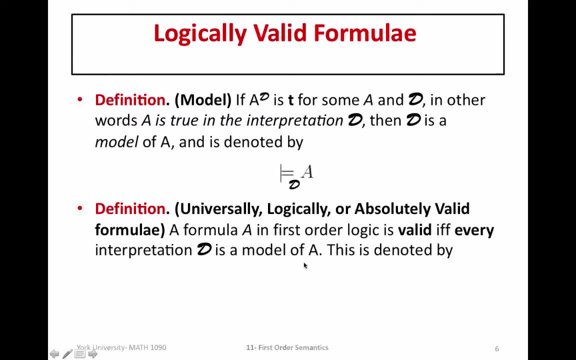 interpretation makes A true, then A is defined to be logically valid, And we denote this simply by models A Instead of specifying the interpretation. we know that every interpretation makes A true and so A is logically valid. OK, so notice that, with this new definition of being a valid formula and these new interpretations, 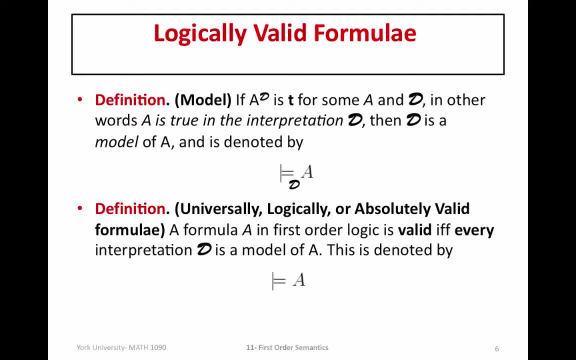 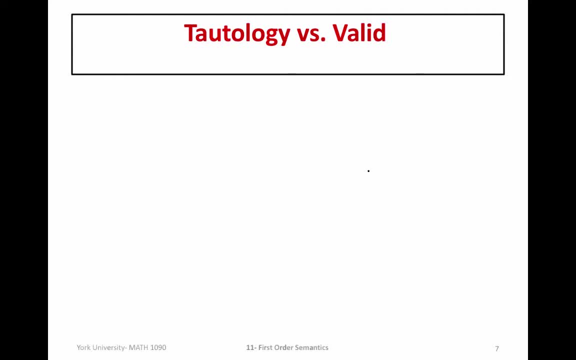 we're defining another way to provide semantic meaning or truth values to first order formula. So we want to compare our notion of semantic meaning previously in terms of tautology with this new semantic meaning of being universally valid or logically valid. Recall that we define a formula in predicate logic to be a tautology if we strip out all. 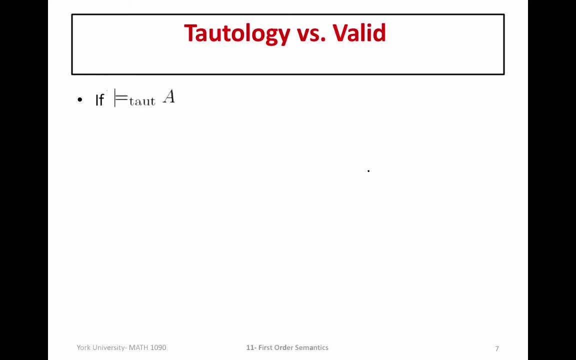 that new meaning, look at its abstraction and look at how the connectives behave in the old way of defining the semantic meaning. So, luckily, if we do all of that and discover that A is a tautology, then it turns out that 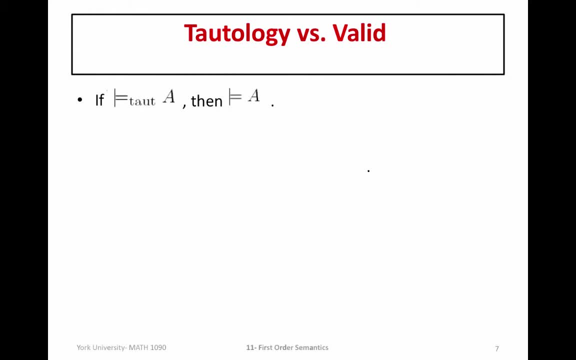 it's a tautology, it turns out that every interpretation of A will also be true. So if A is a tautology, then it's also valid, which is good. However, on the other hand, being valid and looking at the truth, value. 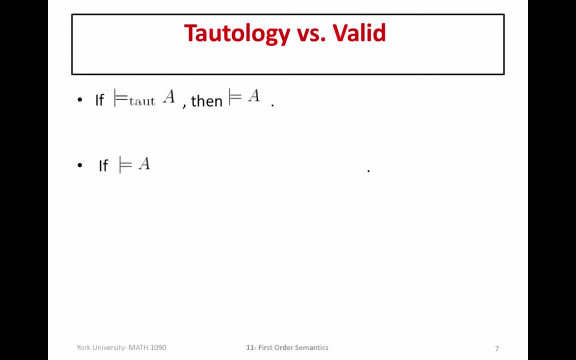 there is a much stronger property because we're not stripping away the meaning of the quantifiers. We're actually looking at what the meaning of that well-formed formula is within particular interpretations. So within any possible interpretation we have, we define A to be valid if any interpretation makes it true. 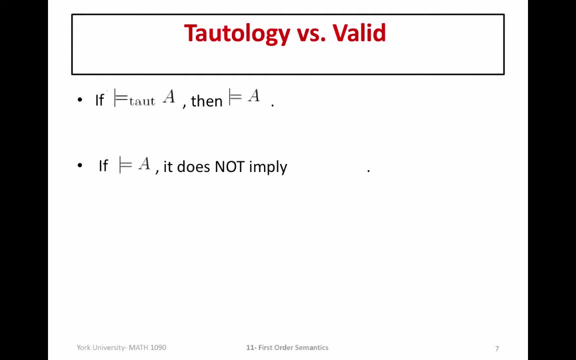 So this is a strictly stronger property, which means it does not imply that A is a tautology, That added meaning provides additional meaning. So, for example, if we consider the well-formed formula x equal to x, we know that, no matter what interpretation we have here, 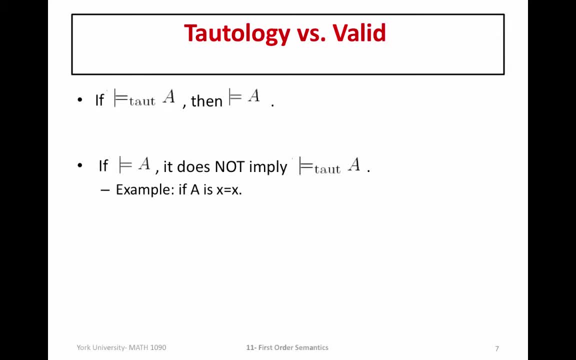 the equal sign has particular meaning that always x is equal to x, right. So no matter how we define our domain, whether it's number sets, whatever equal sign is defined so that x is always equal to x. So that means that this is a universally valid formula. 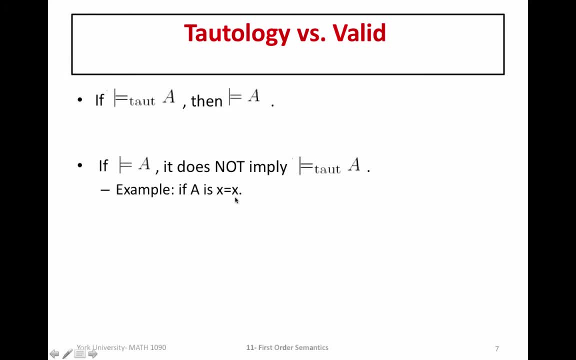 However, it's not a tautology right. Consider what is the abstraction of x equal to x. It's simply the boolean variable p, But there is a state that makes p false, and so that makes this not a tautology. yet it is valid. 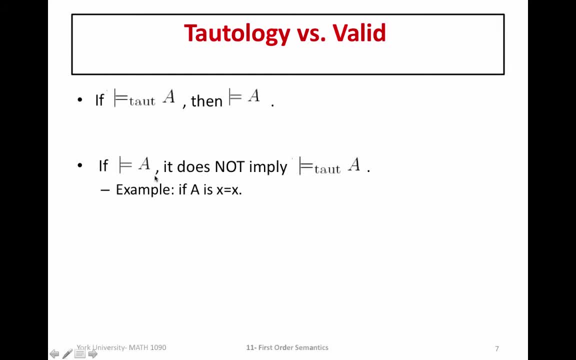 So this provides us with a stronger sense of how to see truth and to, as you will see, construct even more absolute theorems. Okay, so, speaking of absolute theorems, right, remember, in propositional logic, soundness and completeness. 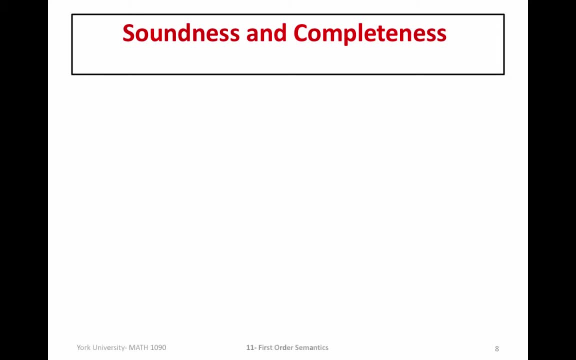 allowed us to connect the meaning of tautology and those semantic truth values with the methods of proofs that we used in our absolute and relative theorems. So now, soundness and completeness within predicate logic involves connecting this new notion of semantics, so this: 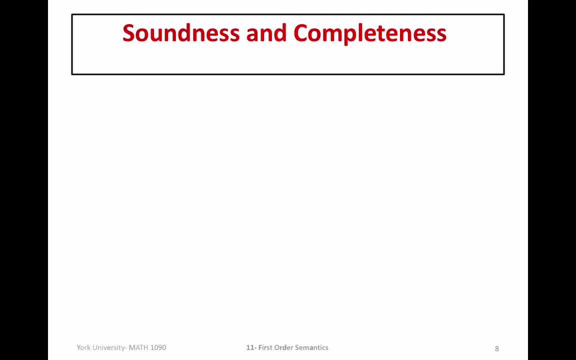 notion of a universally valid formula with ones that are absolute theorems or relative theorems. So soundness in first-order logic says that if A is an absolute theorem, for example, then A is logically valid. So it turns out that everything we can prove is true is: 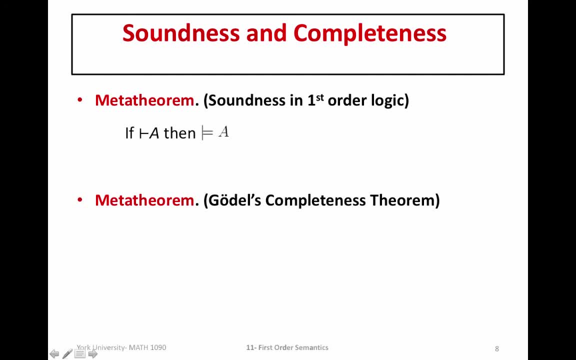 really true. in predicate logic We also have Gödel's completeness theorem, which tells us that predicate logic is also complete. so this gives us the opposite direction. So if A is a universally valid formula, then it can be proven. Okay, notice that to show something is universally valid is actually quite difficult.